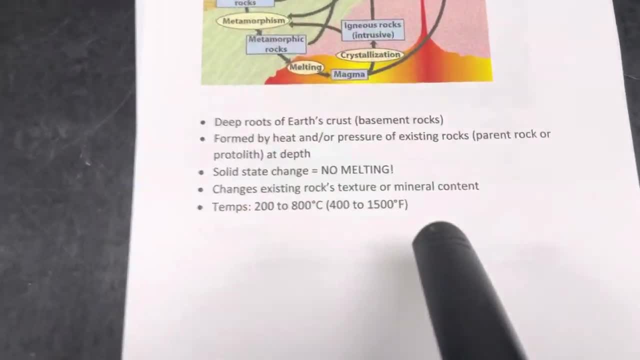 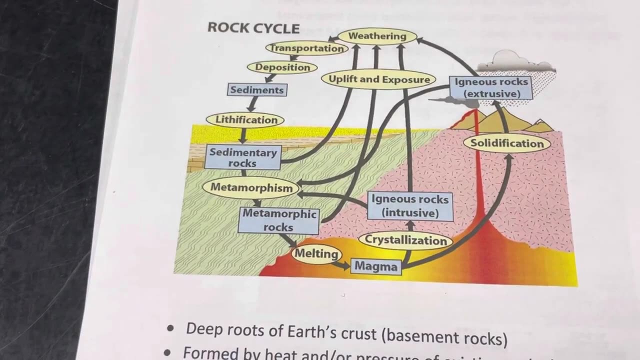 information here, but we will also look at some specific rocks as well And, of course, with our subsequent videos we'll be looking at more rock types in person, which will undoubtedly be helpful to you. So, if we look at some specific rock types, we'll be looking at more rock types in person. 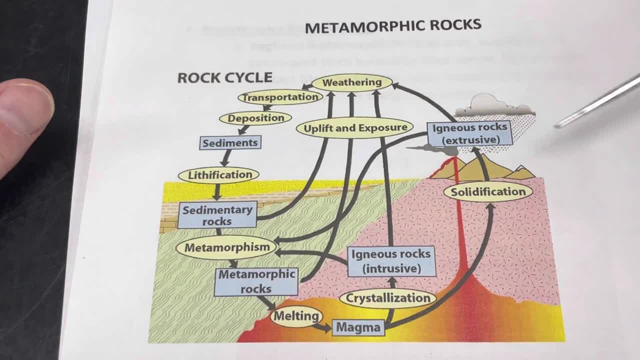 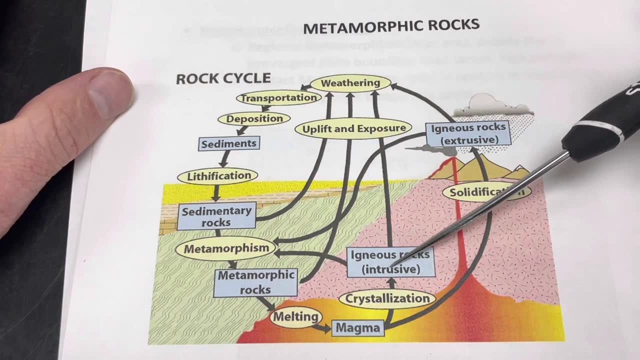 come to the rock cycle, which is kind of where we started our whole exploration of rock types. with the beginning of this series We've covered igneous rocks, both intrusive magmas that cool deep within the earth and extrusive magmas that rise to the surface erupt as lava or ash. 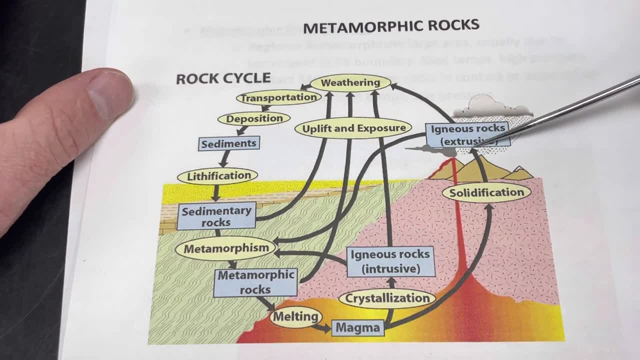 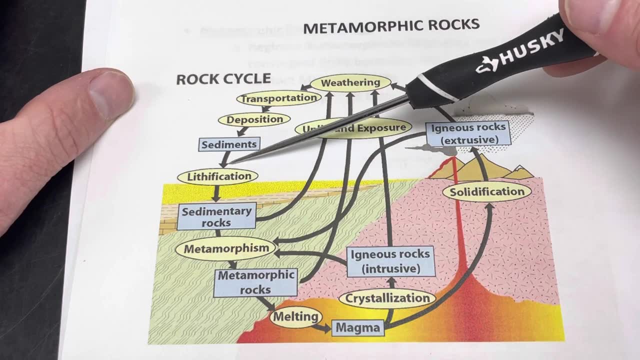 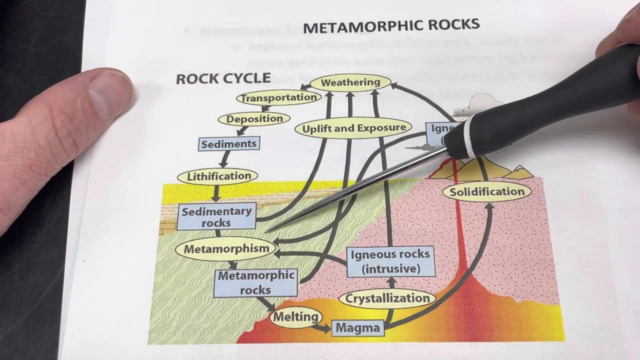 or other materials to form extrusive igneous rocks, volcanic rocks. Rocks get exposed and broken down into particles we call sediments. They can eventually be deposited and buried And brought together to form sedimentary rocks. And we're looking here today and in this video at 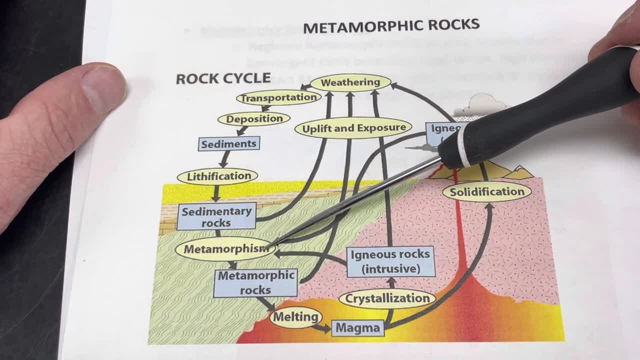 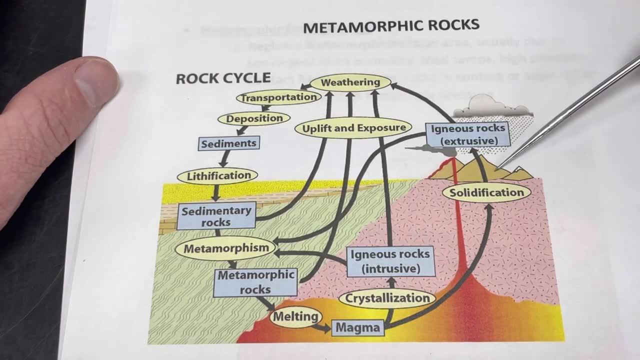 metamorphism and metamorphic rocks. This is kind of a hard concept and area of the rock cycle to wrap your head around because it doesn't take place at the surface. It's not erupting from a volcano, Much like our intrusive igneous rocks. these processes we're going to be exploring. 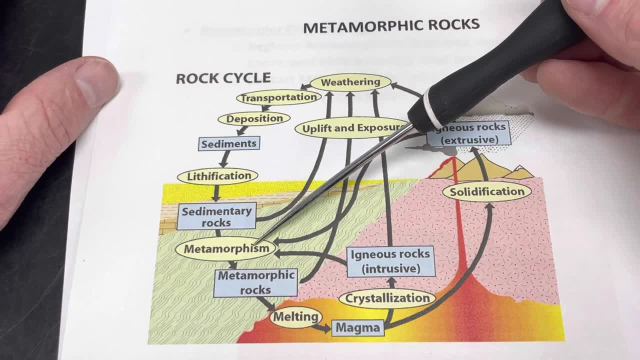 are taking place miles below the earth's surface, where pressures and temperatures are elevated, And so this is a little bit trickier. This is a concept to explore. Notice that the igneous rocks, both intrusive and extrusive, and the sedimentary rocks, all the little arrows in the rock cycle here, bring you to metamorphism. So 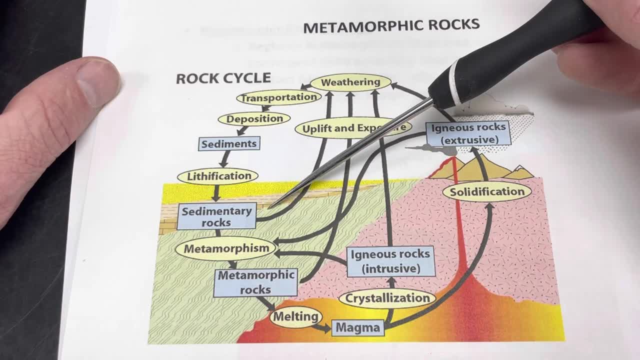 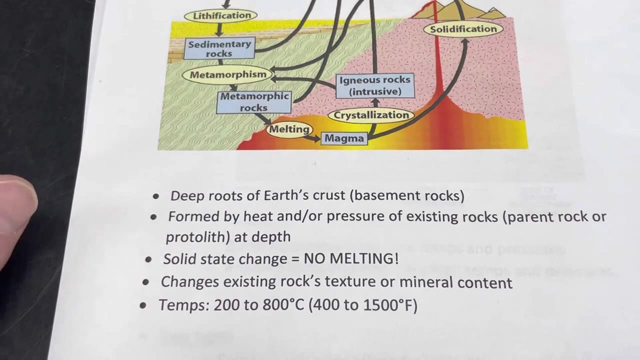 that tells us that any of these given rock types, given the right sort of conditions, can be buried deep enough where they are subjected to the high temperatures and pressures that produce metamorphism. So let's move on and a couple other important points that we'll make here as we go. 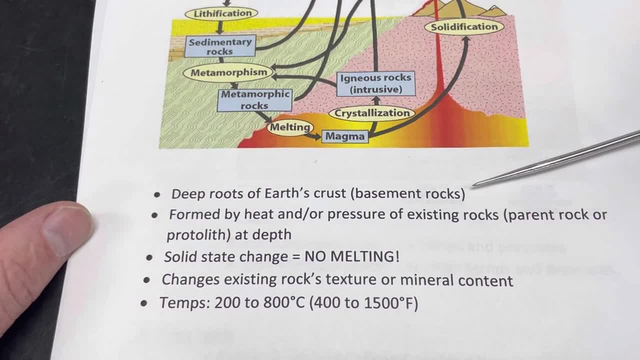 along, So metamorphic rocks tend to form what we call the basement rocks, the very deep roots of our earth's crust. deep below the mountains, Even wherever you're standing, miles below your feet, there are metamorphic rocks. So these rocks tend to form the- a lot of times, the oldest rocks in. 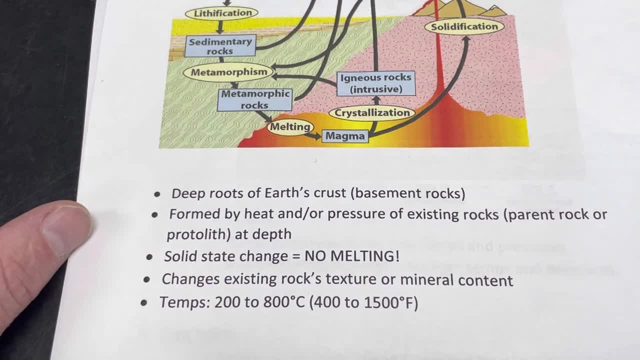 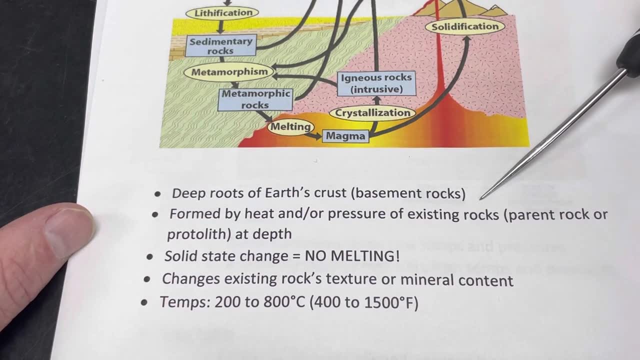 the crust and also the deepest rocks, As we talked about, heat and pressure are the big driving processes here. So we're going to take existing rocks, any type of existing rock, and we call that rock that exists in the air before it became a metamorphic rock. we call that either the parent rock or another term. you. 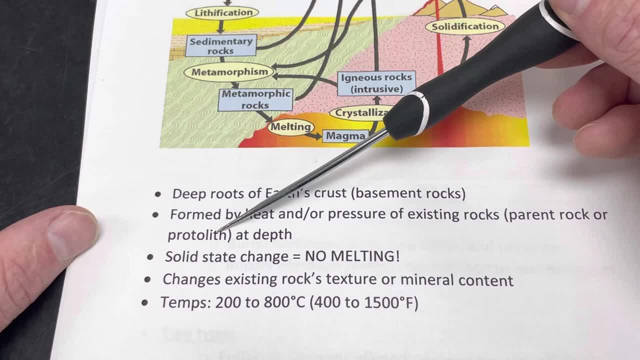 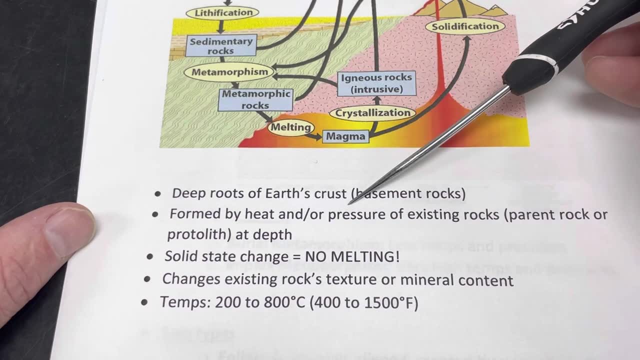 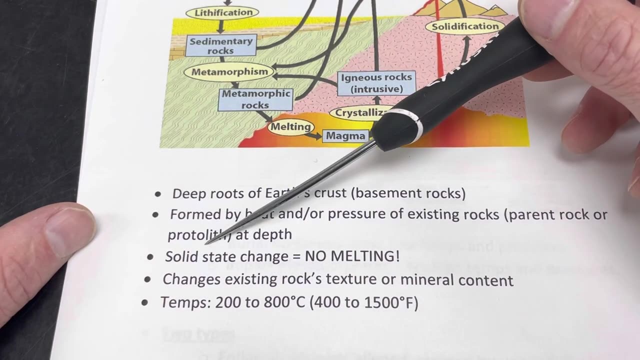 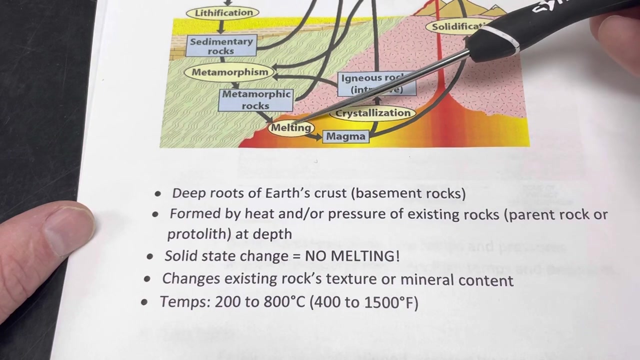 sometimes hear, is protolith, so before. so the parent rocks can be any existing rock and again, subjected to high enough temperatures and pressures, those will change into metamorphic rocks. this is an important point here. metamorphism is a solid state change. it does not involve melting. remember here, if we look at the rock cycle, if you completely melt a rock you are back to magma. 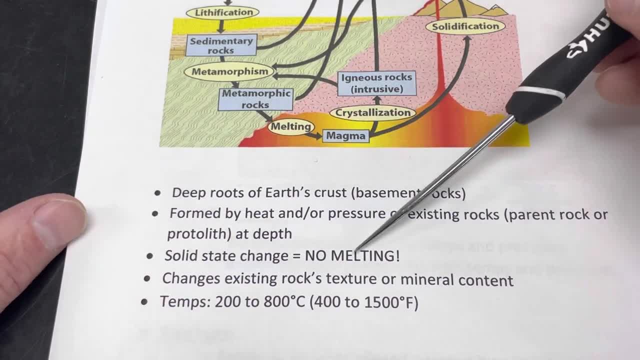 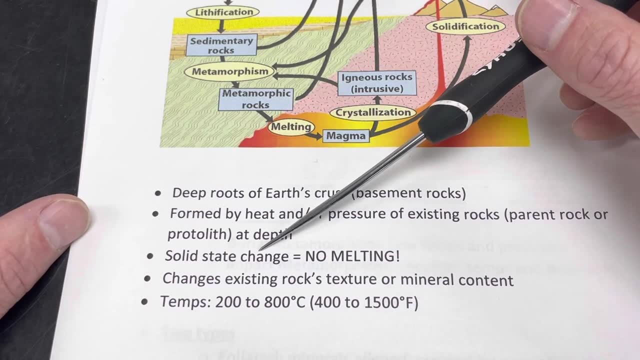 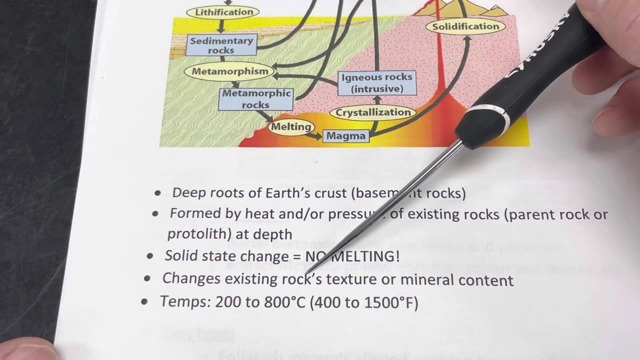 and then you're back to the igneous part of the rock cycle. so metamorphism is a solid state change. we are not melting the rock. there may be some tiny bit of melting- that's possible with some of our higher grade metamorphic rocks- but basically we're changing the rock's texture or the minerals that 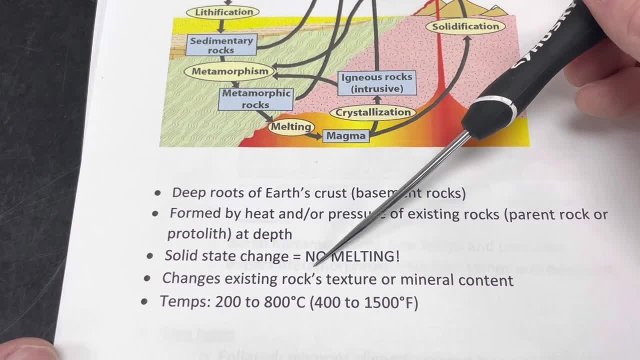 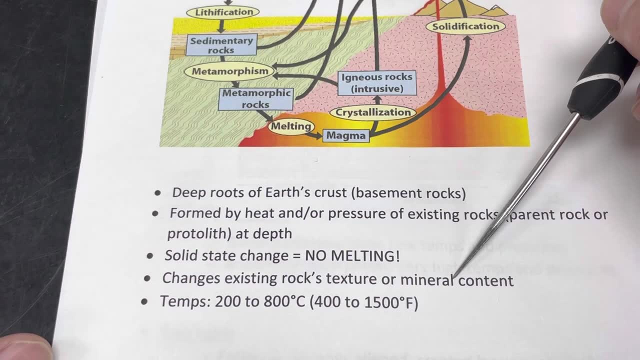 make up the rock by the presence of heat and pressure. it could be that the rock's being squeezed in a certain way. it could be that the minerals that the rock was originally made of are no longer stable at the higher temperatures and pressures, so they break down and the elements 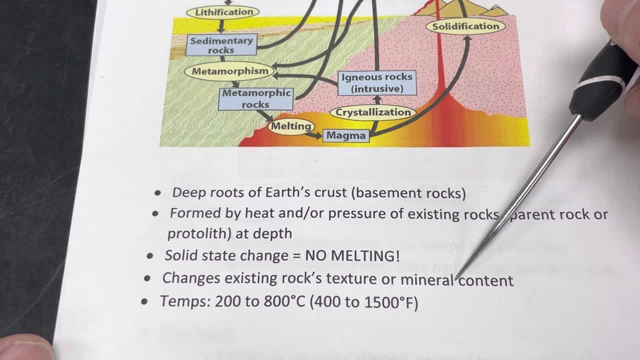 recombine to form new minerals that are stable at those higher temperatures and pressures. and then these are. this is sort of the temperature range we're looking at here. so what does it take to metamorphose a rock in terms of actual temperature measurements? you know we're. 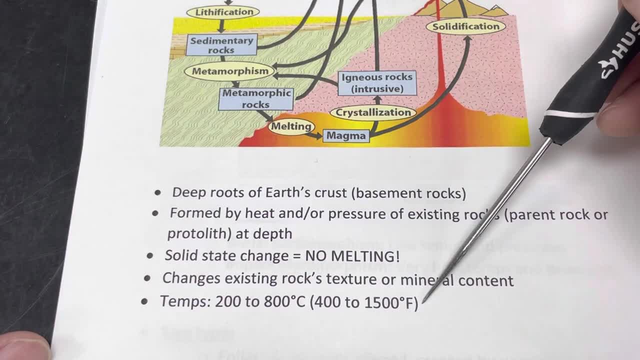 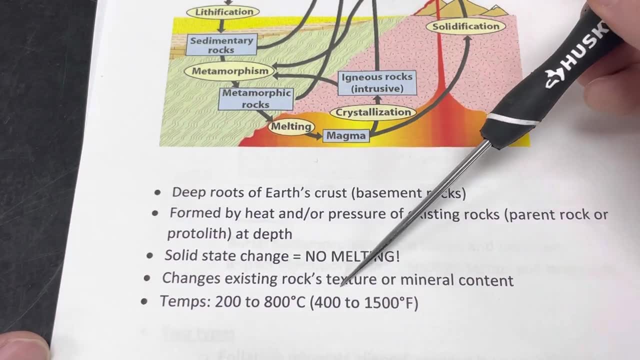 looking at two to eight hundred degrees celsius, four to fifteen hundred or so degrees fahrenheit, you exceed these numbers here and again you're back to melting. why is there such a big range here? well, it depends on the the original material, depends on what the original rock type was. 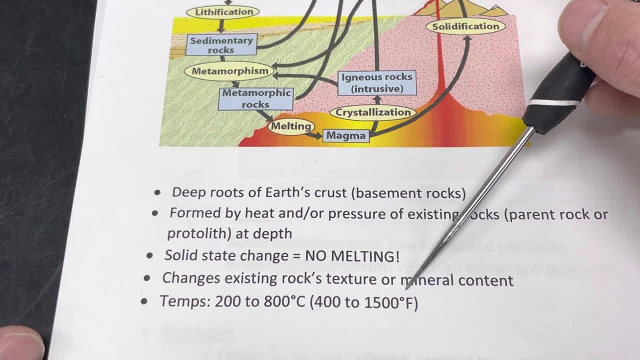 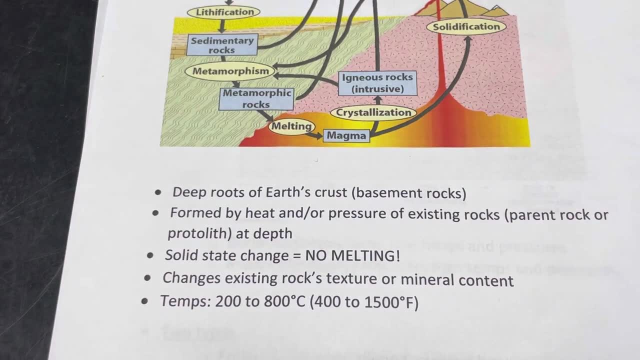 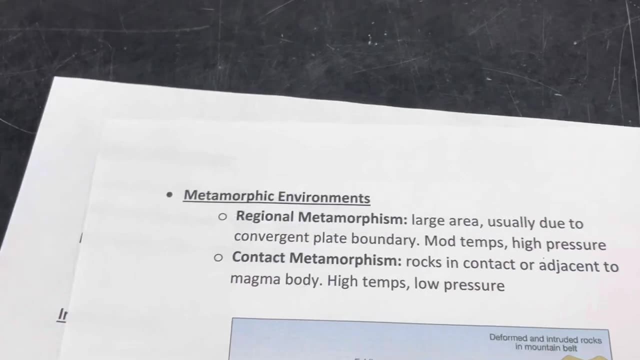 what its mineral composition was and some other factors that sort of dictates this. but this is the sweet spot. this is the temperature range at which most rocks will undergo a change that we call metamorphism. so let's go to where we actually see this type of thing taking place. 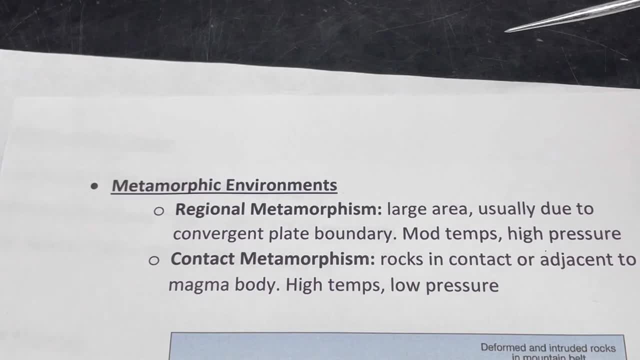 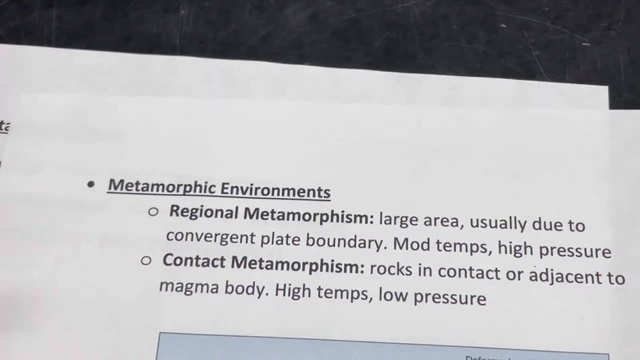 what are some of the environments. so we're going to go over a couple different situations where rocks can become metamorphic rocks. the first one we'll look at here is what we call a regional metamorphism, so this usually takes place over a big area, like a lot of times it's. 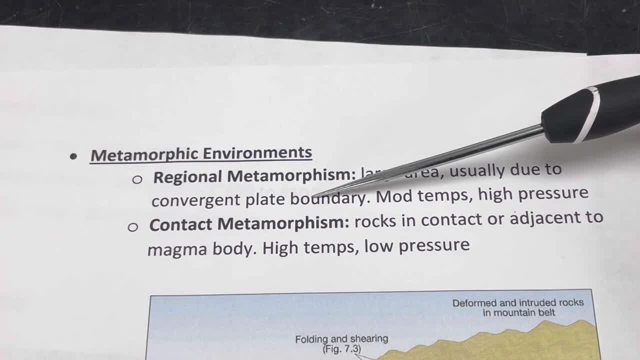 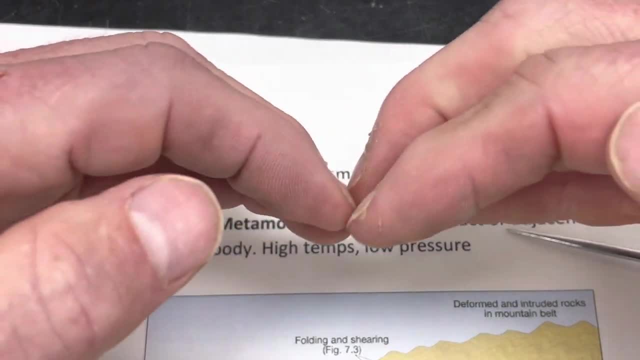 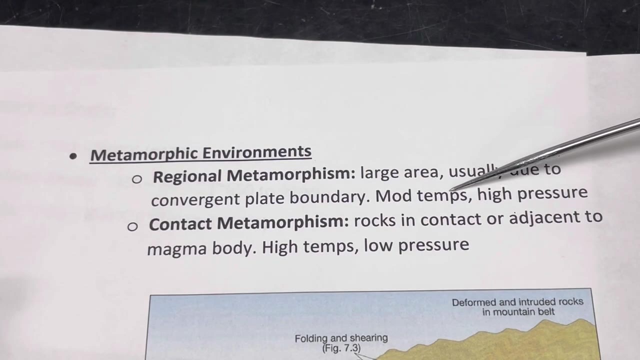 related to a convergent plate boundary, where the two plates are colliding and slamming into each other. as those two plates are brought together, the rocks in between are being squeezed, and so we would tend to get fairly high pressures, but maybe not as high temperatures. in terms of how elevated those temperatures are, maybe more like. 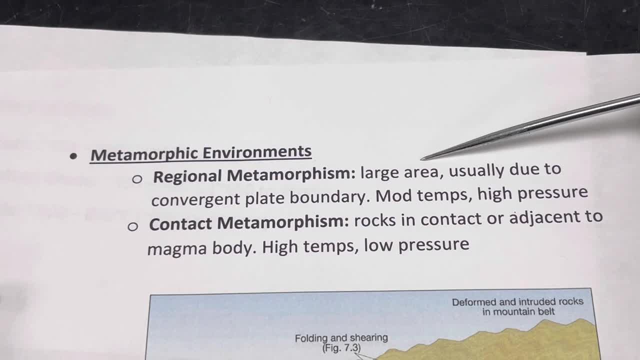 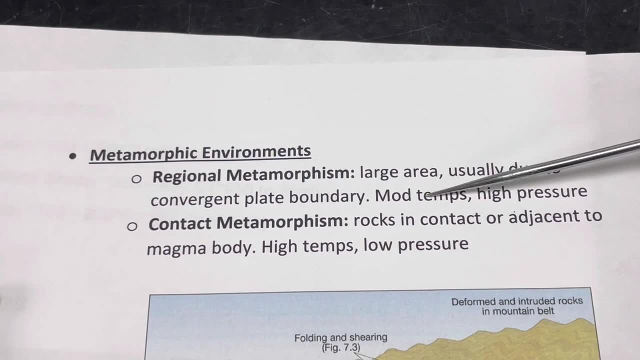 moderate temperatures. so regional metamorphism will change rocks into metamorphic rocks over considerably large area. where might we see this today? well, if you think about india and its continuing collision with asia, which is forming the himalayas, the big mountain chain. at the surface, deep under the roots of those mountains, we could surmise that the temperatures are high enough. 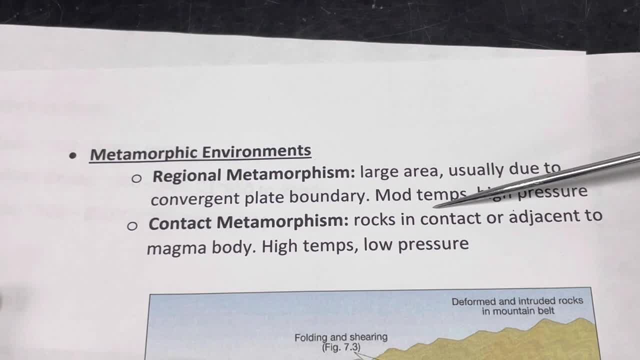 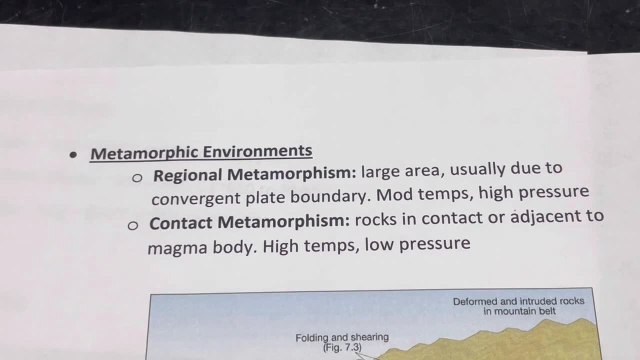 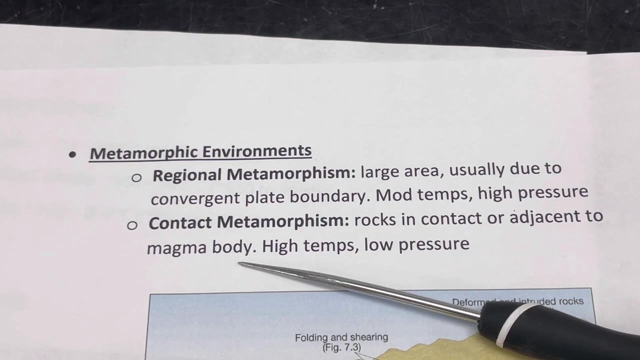 and the pressures are intense enough that those rocks are being changed, even as we speak, into metamorphic rocks, and we'll look at the effects of that squeezing here in a minute. another type of metamorphism that's possible is if you have some, uh, subterranean magma body, so a magma chamber or magma that's. 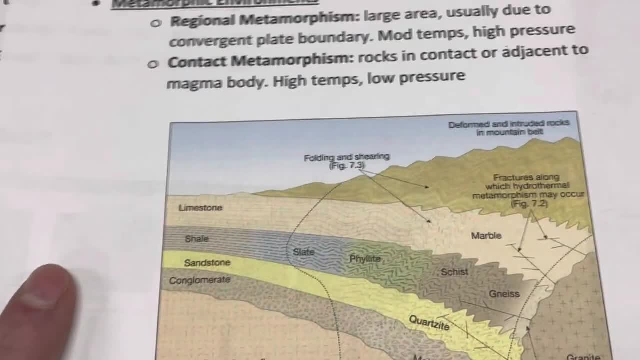 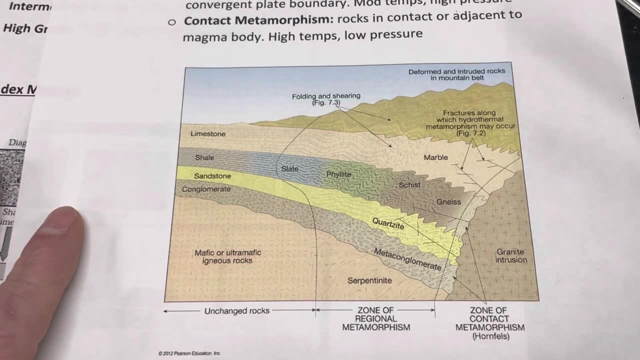 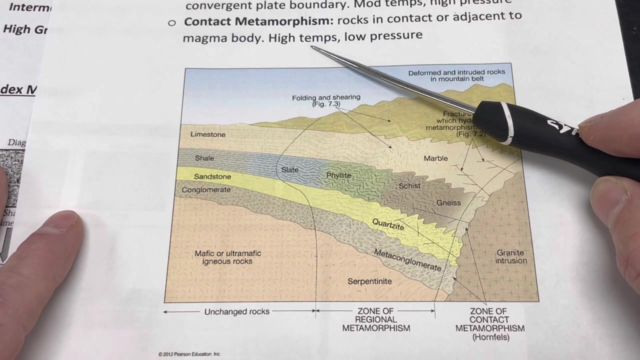 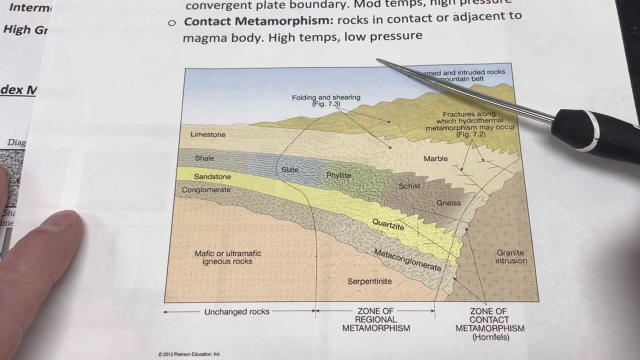 in the subsurface, the rocks that are touching that will tend to form um metamorphic rocks, and that's what we call contact metamorphism, and so this tends to fight against some of these rocks And so this tends to form very high temperatures because you have magma which is upwards of, you know, 15,, 16,, 1700 degrees Fahrenheit, maybe something like 1000 degrees centigrade, but relatively low pressures because a lot of time the contact metamorphism takes place at fairly shallow levels of the Earth's crust. 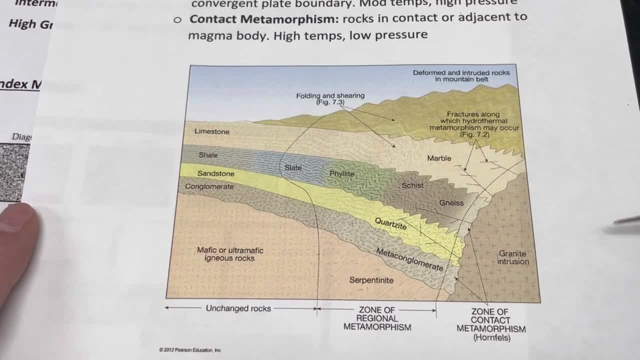 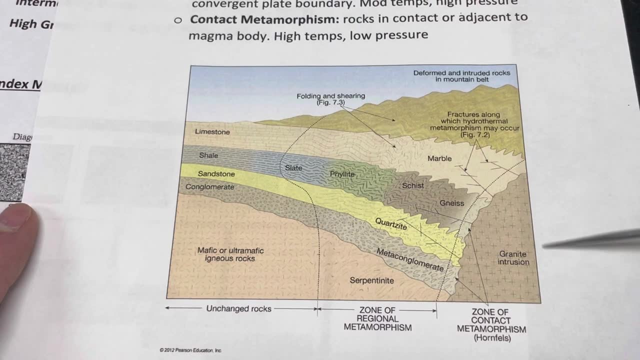 This diagram here shows what you might see, and there's a lot going on here. So this down here in the bottom right corner, this is the magma body. So this is where the magma was in contact with the surrounding rocks, And so what we might see is this magma cools into granite. While this magma was still molten, it's changed. the existing rocks, The limestone over here in proximity to the magma, has been changed into marble. 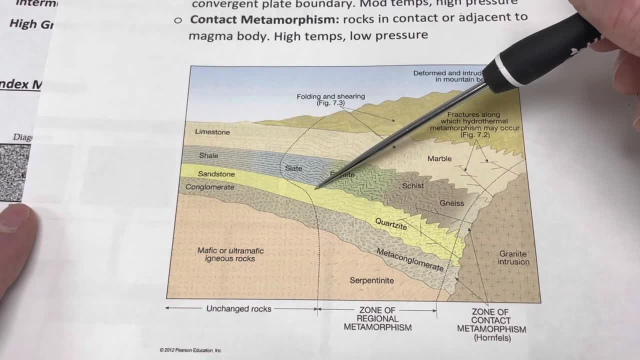 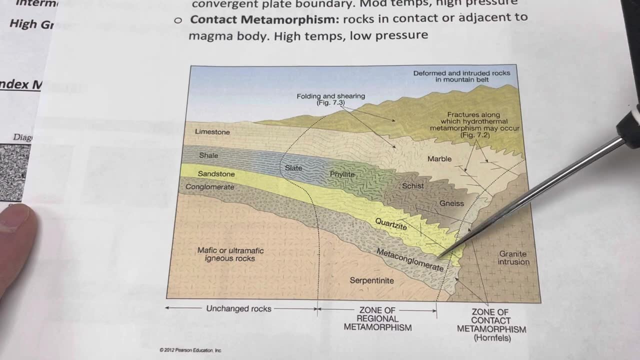 The sandstone over here As you get closer to the magma body and the heat source, has been changed into a metamorphic rock called quartzite, And you can see that with some of these other rock names as well, which which we'll get to. 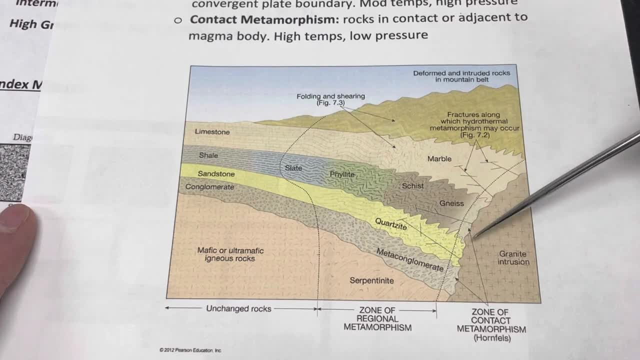 So there's a whole host of rock names in this sort of metamorphic zone adjacent to this magma body. But this would be a good example of contact metamorphism, where the magma body is in contact with the pre-existing rocks and the heat from that magma body, along with circulating fluids and maybe some other processes. 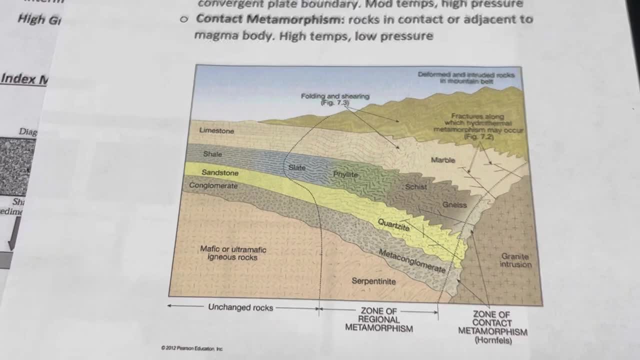 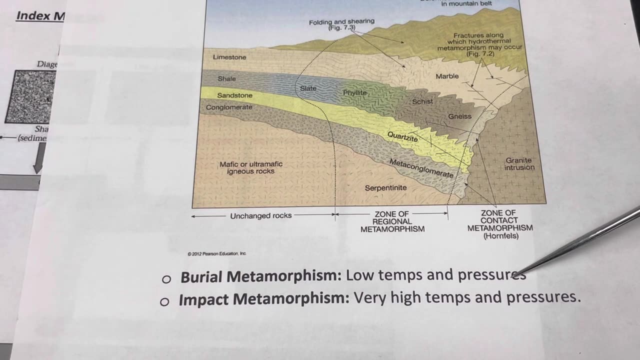 So these reg gear will move as before and will change the rocks over time into metamorphic rocks. What are some other environments where we might get metamorphism? Well, you can just bury rocks, right. So if you just bury sediments or deposits deeper and deeper and deeper, eventually you can bury those materials deep enough that the temperatures and pressures are high enough that you're starting to enter that metamorphic realm. 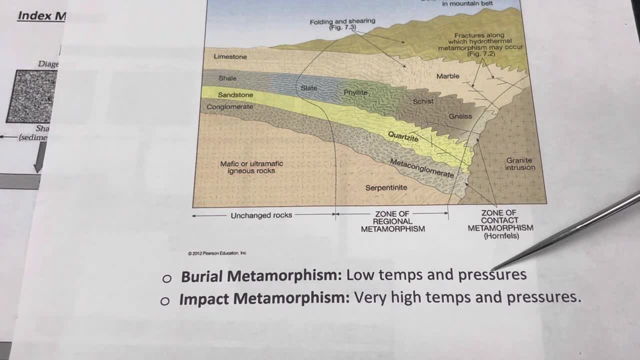 And so burial metamorphism. we might not expect super high temperatures or pressures, but there are enough many times to cause changes in the rock and become metamorphic rock. So here is the question: what happens when this Release Of The Rock Dad Mode is removed and there are no changes? 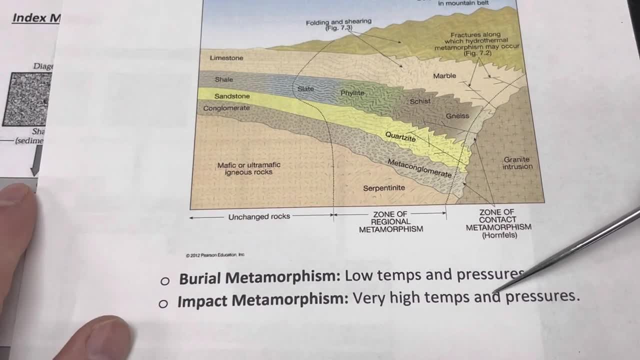 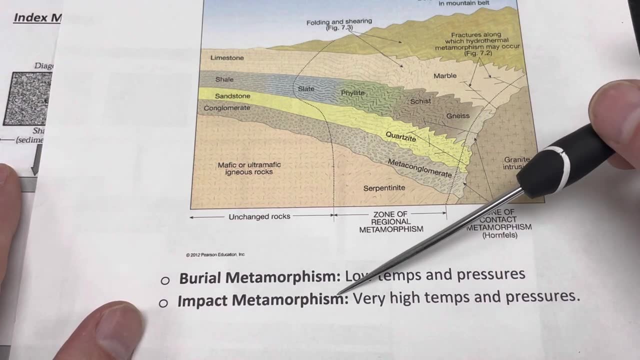 metamorphic rocks. and then this last one here doesn't happen very often but it's fun to think about, kind of a exciting and sexy situation and that's impact metamorphism. so if we have meteorites smashing into the planet, the speed of those meteorites combined with their, their density, 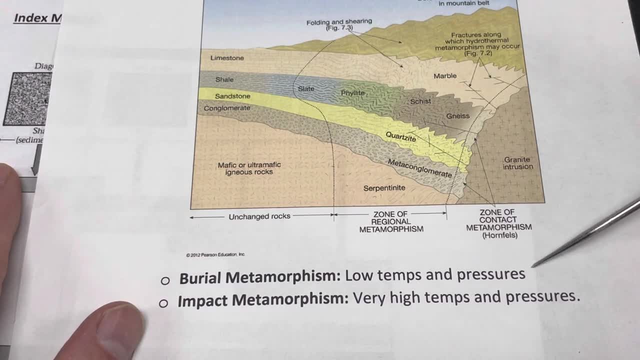 and their mass produces extremely high temperatures and pressures on the rocks that they run into and you can get some interesting minerals and textures and features in these rocks. so this is what we call impact metamorphism- definitely not as prevalent as the three we just covered, but it's. 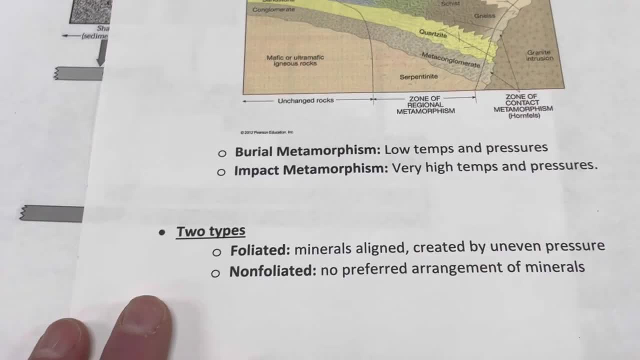 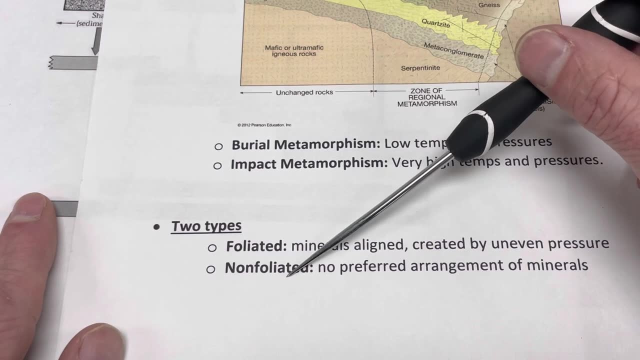 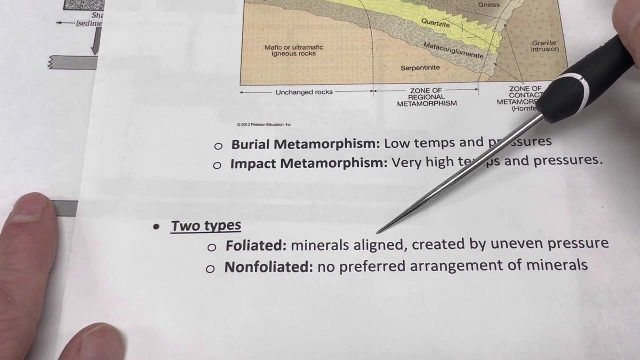 fun. it's a fun one to talk about and think about a little bit. okay, so metamorphic rocks are going to be of mainly two types. they'll either be foliated or non-foliated. and what does that mean? well, foliated means that the minerals are aligned, that the the rocks have been squeezed. 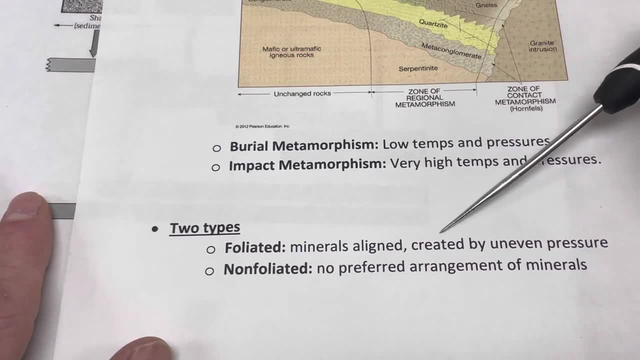 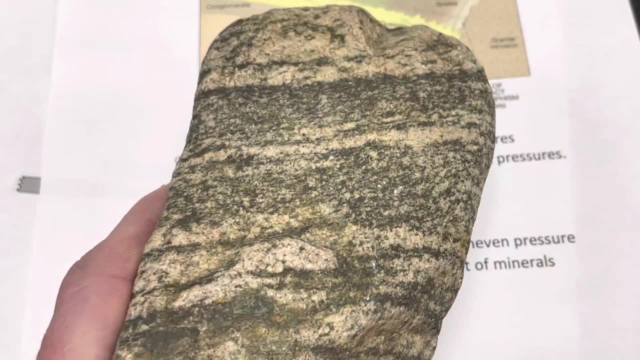 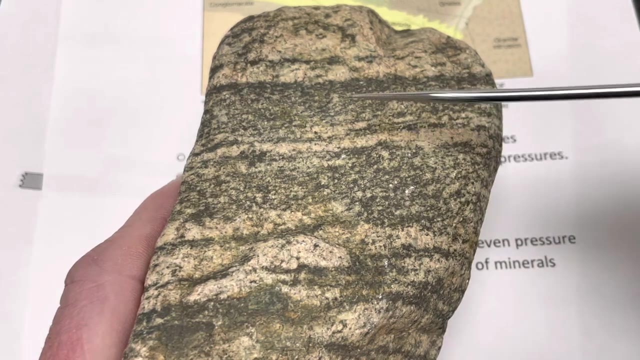 probably due to regional metamorphism or uneven pressure, and the minerals are aligned, and so here's an example of how that might look in an actual metamorphic rock. this is a metamorphic rock called gneiss g-n-e-i-s-s, and we can see the obvious banding or layering in these crystals. 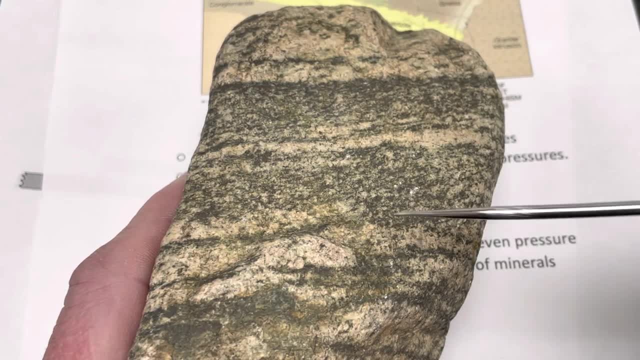 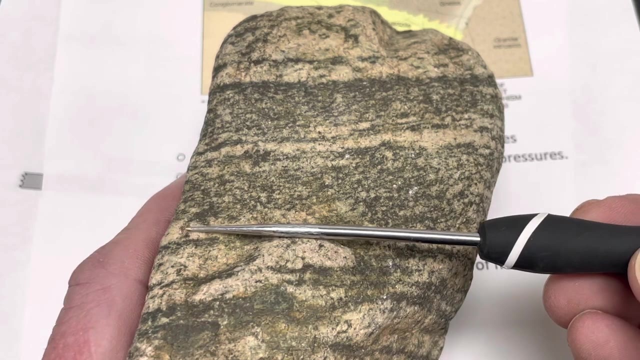 in this metamorphic rock, what the these minerals define is a textural feature called foliation, so this is definitely a foliated metamorphic rock, and this is an example of how that might look in a metamorphic rock, because the minerals are aligned in a planar or semi-planar fashion. 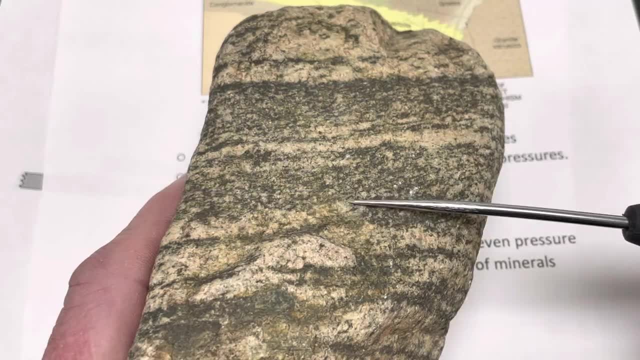 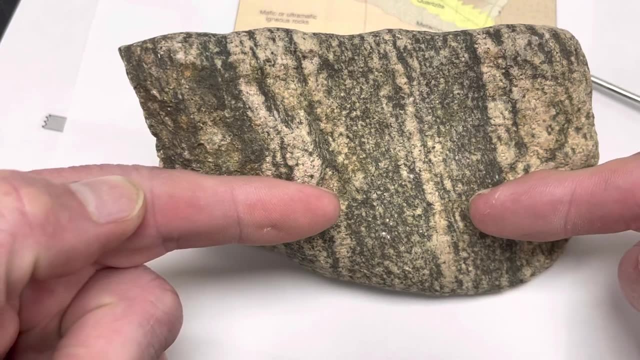 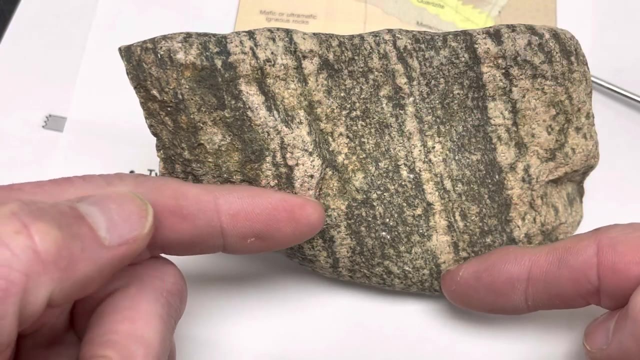 defining this foliation texture. what we could then surmise, then, is that this rock has been squeezed on either side in this direction in order for the minerals to line up perpendicular to that. so we can look at the orientation of the foliation and then estimate that the pressure, the uneven pressure, 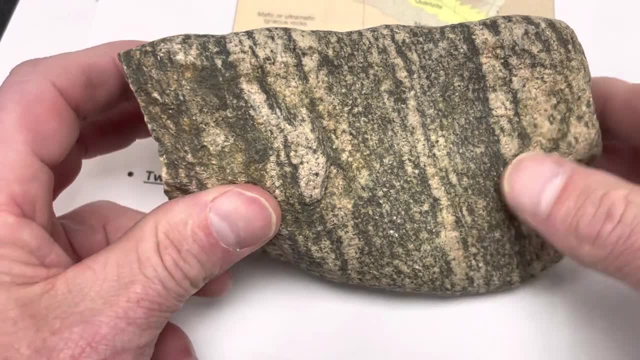 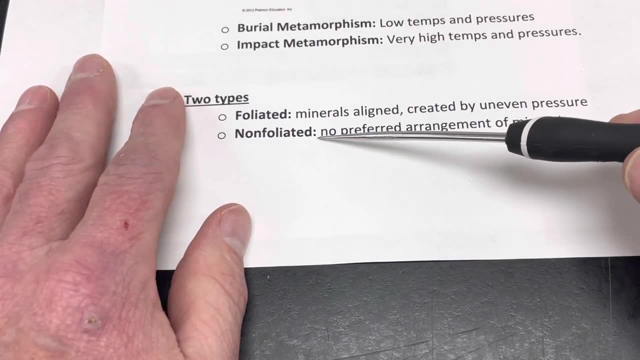 that's going to be applied from a perpendicular direction, perpendicular to the foliation direction there. what we also sometimes see, though, if we don't see a preferred arrangement of minerals, that's just called non-foliated rock, so the rock may be squeezed and the crystals are kind of dense. 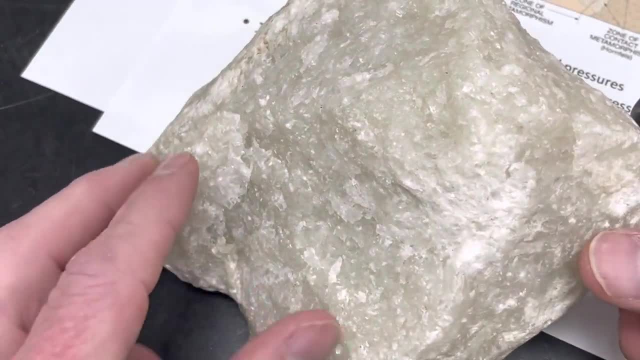 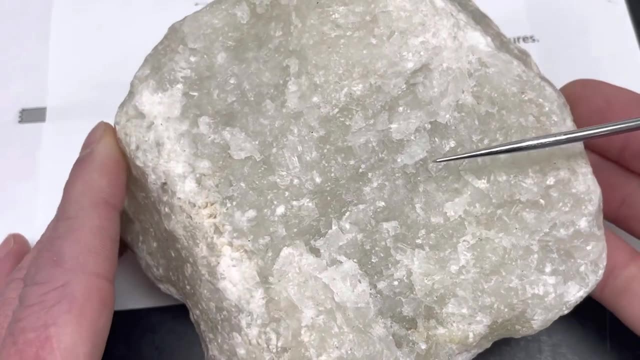 but we don't see a preferred orientation of the minerals. so this is a nice piece of marble and you can see that it's crystalline. if we rotate it in the light you'll see some sparkles in there. this is totally made out of calcite. 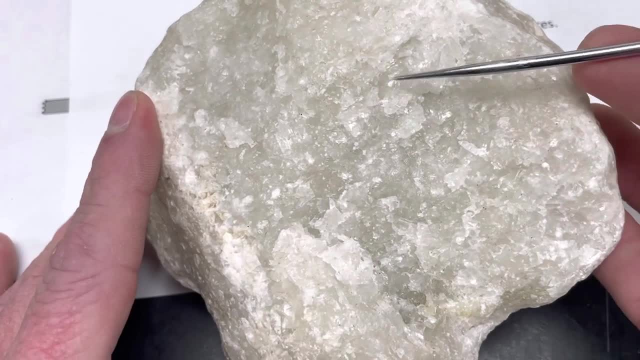 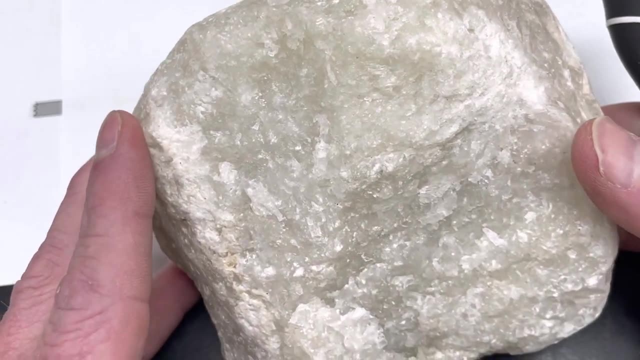 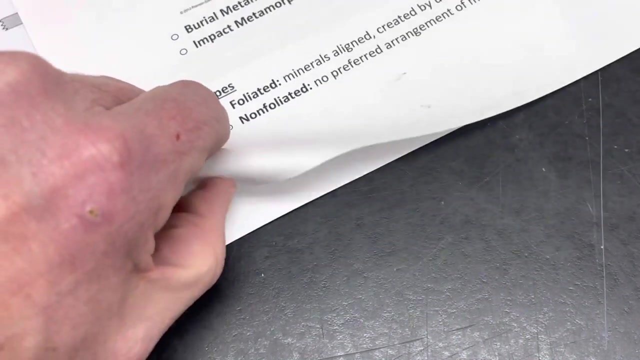 you can see with the mineral crystals in this metamorphic rock that they're kind of randomly oriented. there's no preferred orientation. therefore, this would be a non-foliated rock with no visible pattern or fabric running through the rock itself. so um so said, uh, um, metamorphic. 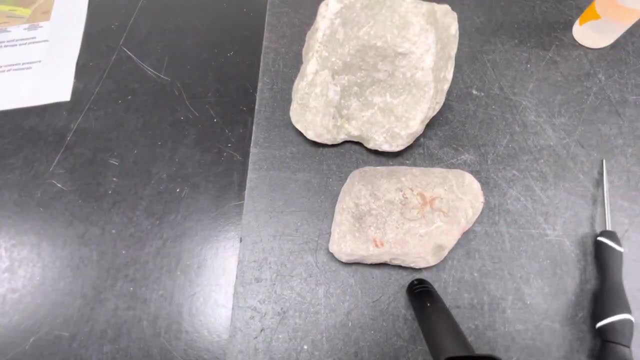 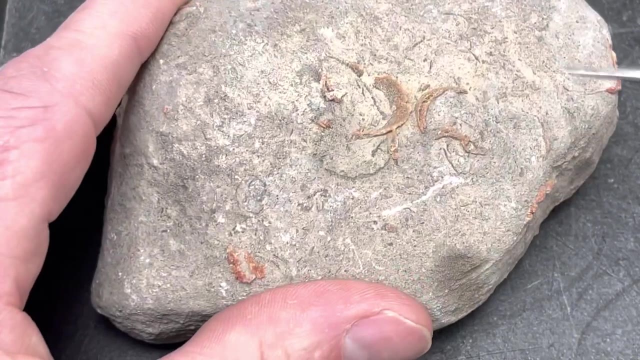 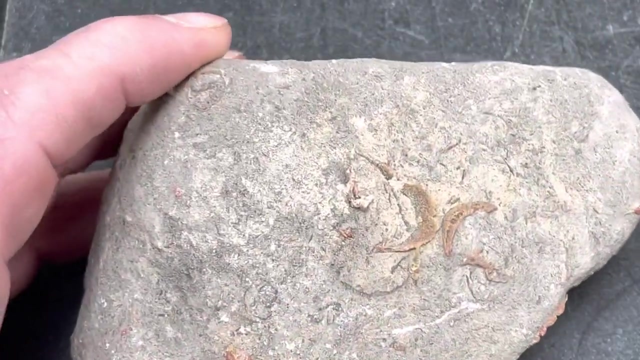 changes can be kind of slight, and let me just kind of illustrate a couple things here. so here, what we have. this rock here is a limestone. you probably can pick out some of the shells. there's some fossils in here. these kind of web looking things are called bryozoans. this is just a really kind of classic limestone. 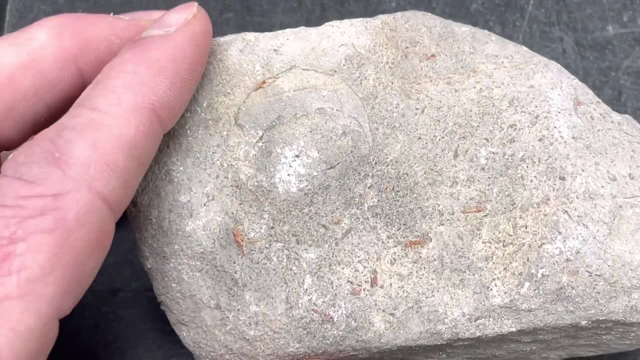 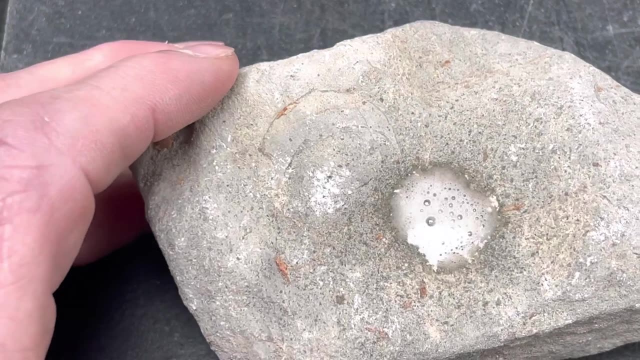 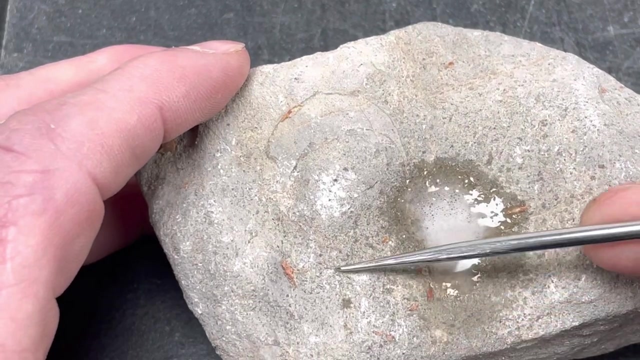 with some fossil material in it. of course, limestones, as we've learned in our series, are totally made out of calcite. so the the main mineral that makes up a limestone is a mineral called calcite. but the calcite here is in the form of organisms, shells and hard parts. 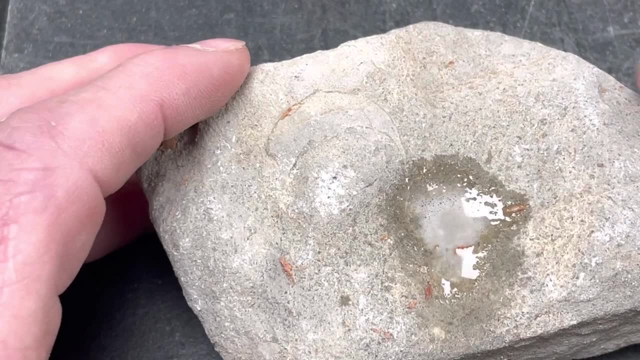 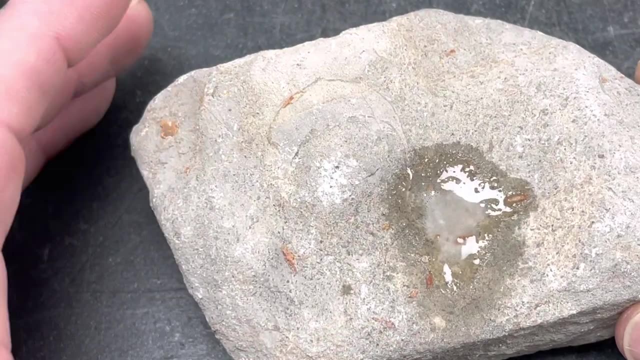 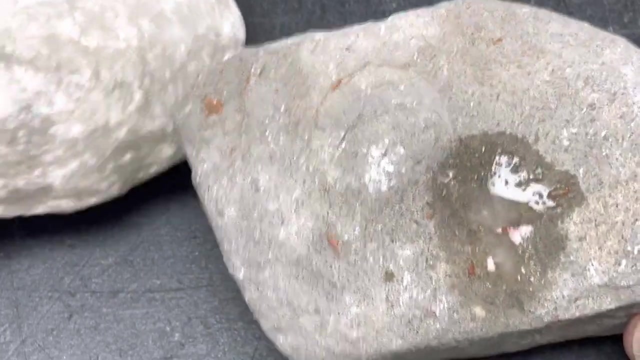 from organisms that have accumulated on the ocean floor and then been compressed and compacted into rock. when this limestone gets metamorphosed, it gets heated, and now it's at temperatures and pressures where these organisms, these shells, um, maybe aren't as stable, and that causes the 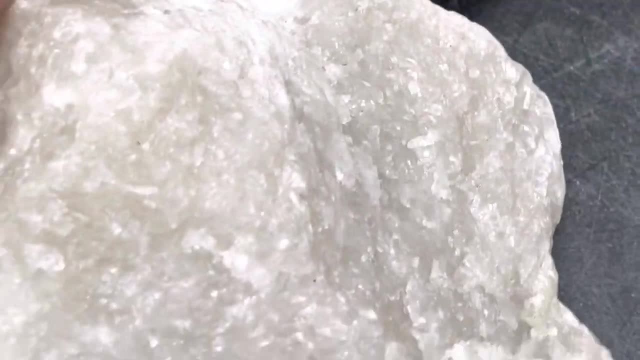 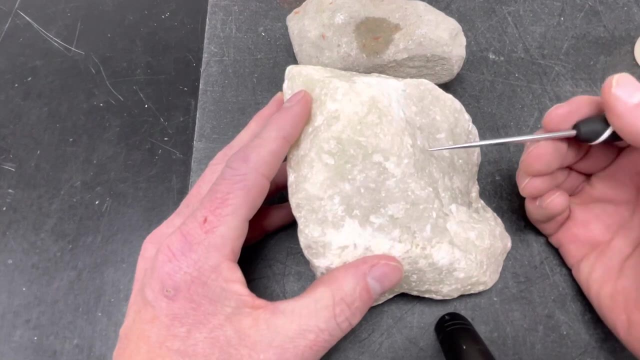 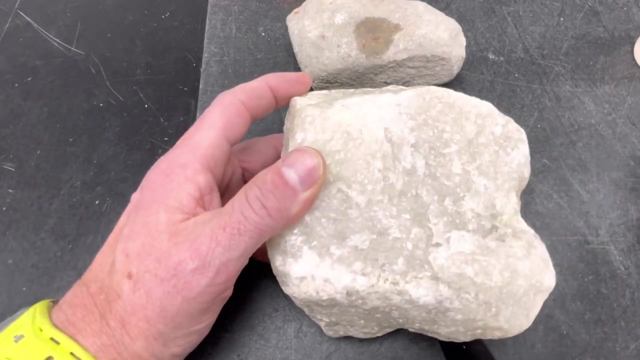 calcite in that to completely recrystallize and form a new rock called marble. but the limestone and the marble have the same composition and ingredients. so the limestone is made out of calcite, this is totally made out of calcite. the only difference here is the calcite has completely recrystallized to form this new rock marble. but if i hit it with 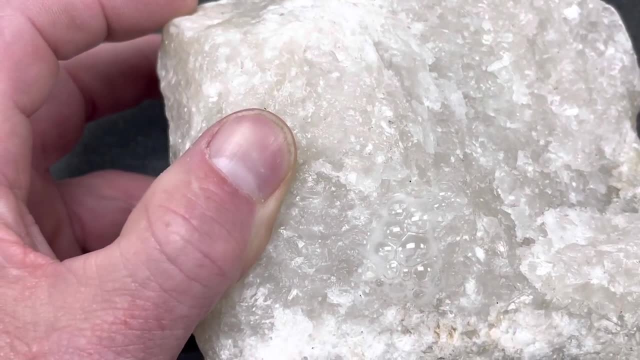 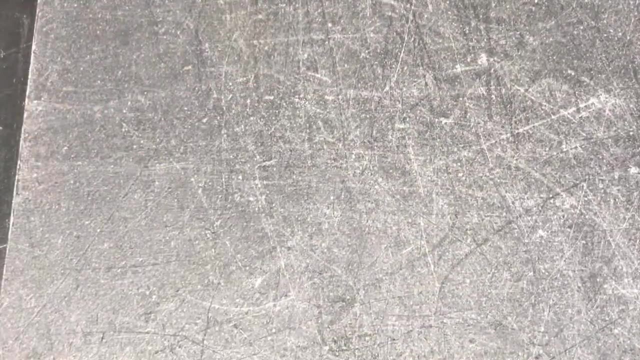 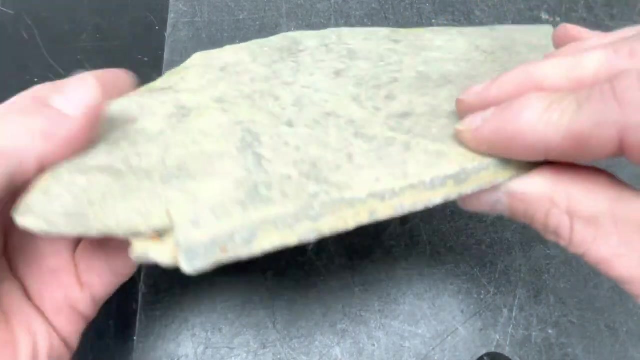 the acid, it should bubble and fizz, just like the limestone does, kind of confirming there that we have the calcite making up the rock itself. another example- because these metamorphic changes can be kind of slight or they can be a little more prevalent- we've got this very thin planar rock. 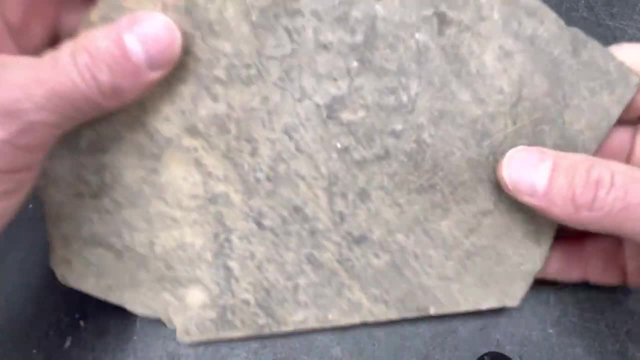 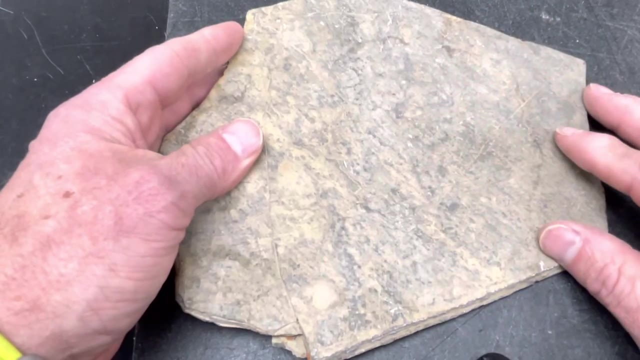 it's very smooth to the touch. i rub this with my thumb. it's very smooth to the touch. this is a sedimentary rock. we've learned this is called shale. it's kind of dull colored. it's fine grained, splits into layers when this gets heated up just a little bit to fairly low metamorphic temperatures. 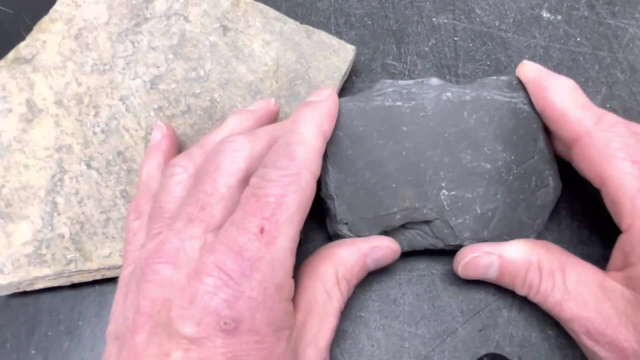 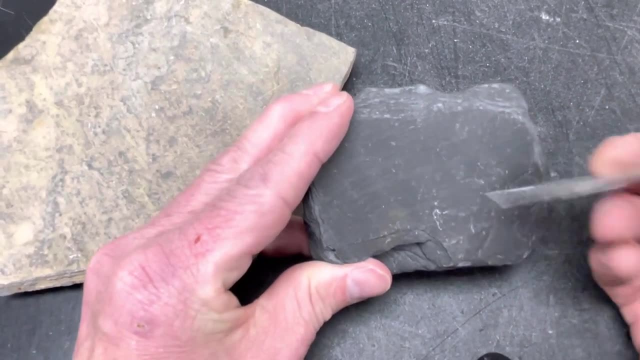 and pressures it can turn into a rock that is also kind of dull colored. this one just happens to be a little bit darker, but it could be basically the same color, but it still has a lot of the same properties. it's fine grained if you look at the crystal size. 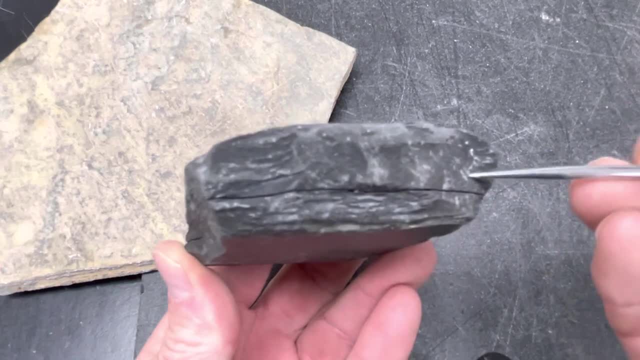 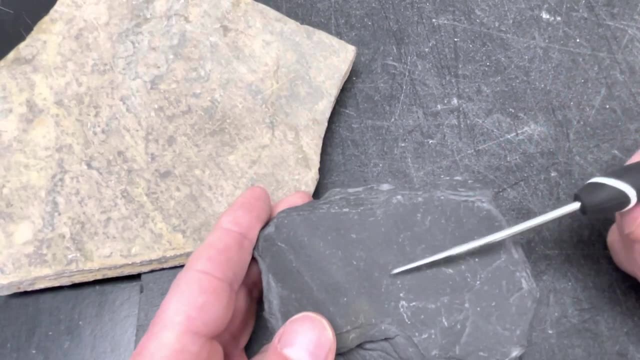 all it tends to break into sheets. looks like it actually wants to break right now along that crack there, and this is a metamorphic rock called slate. so in this case, the shale to the slate change as we increase the temperatures and pressures. a little bit doesn't seem to be that. 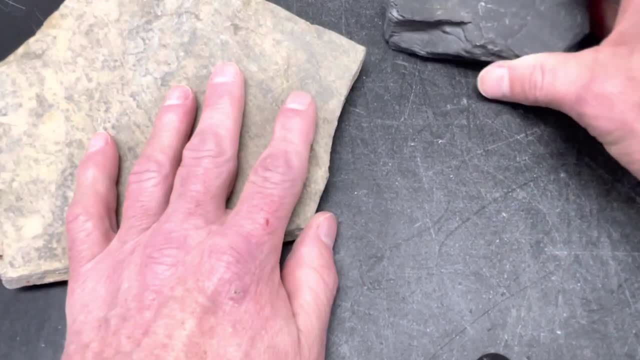 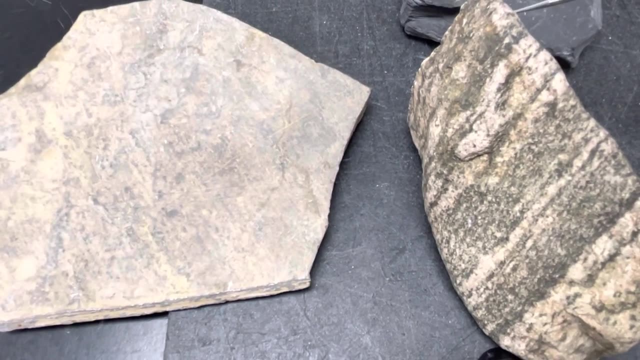 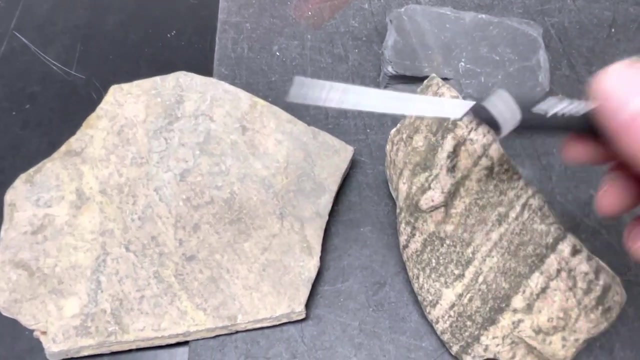 drastic. but if i take this same shale and exert even higher temperatures and pressures on it, i could get something like this nice. so this nice and this slate here has the same parent rock shale. so those two rocks share possibly the same parent rock. the only difference here is the amount of 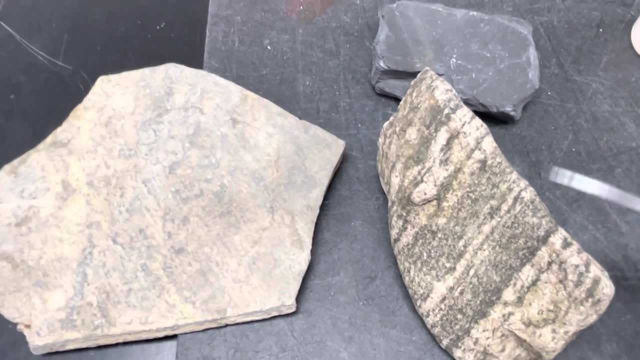 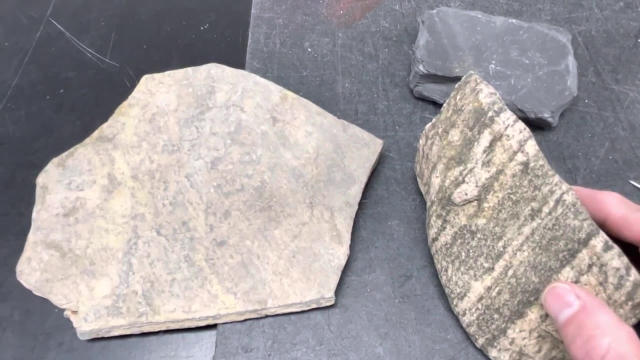 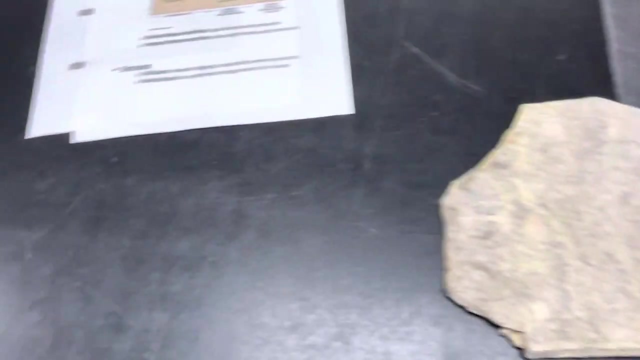 temperatures or the the elevation of temperatures and pressures. this is a high grade metamorphic rock. this rock forms when shale or other rock types are subjected to very high temperatures and pressures. so notice that metamorphic changes can be pretty dramatic, or they can be a little more subtle and a little bit more slight. okay, so our last little bit of uh info here, if you're. 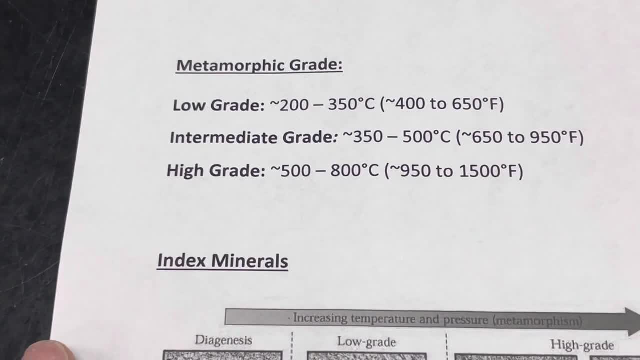 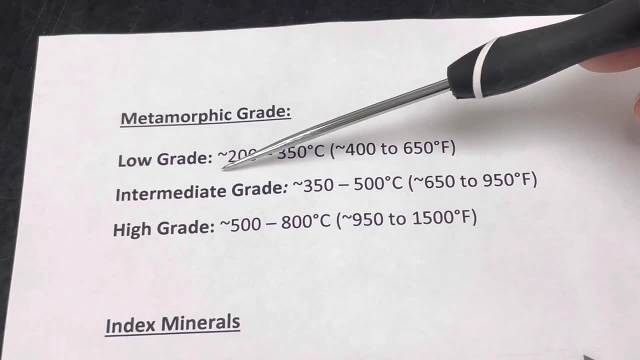 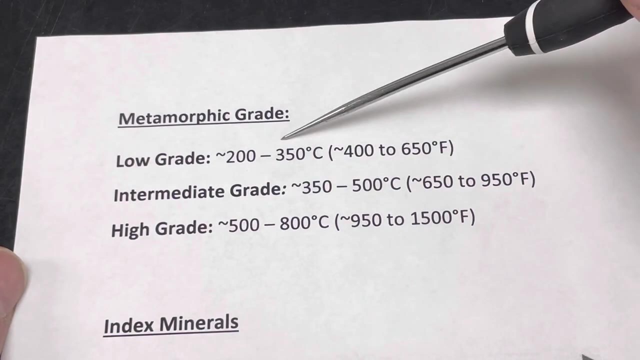 hanging in here with me- and i hope you are- is um, a broad classification of just metamorphic grade. we sometimes, out of convenience, refer to the temperatures that the rock was subjected to by using either low, intermediate or high grade metamorphism. and these numbers here are just a. 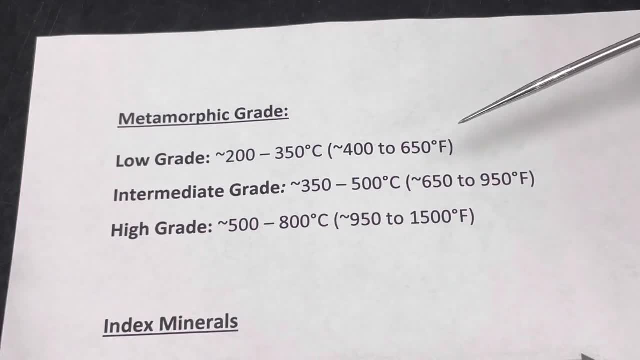 pretty good approximation of the temperatures involved. now a good question to ask would be like: well, how do i know? let's say i've found a metamorphic rock. i feel good that it's a metamorphic rock, but i have no idea if this rock is a low, intermediate or high grade. in other words, i have 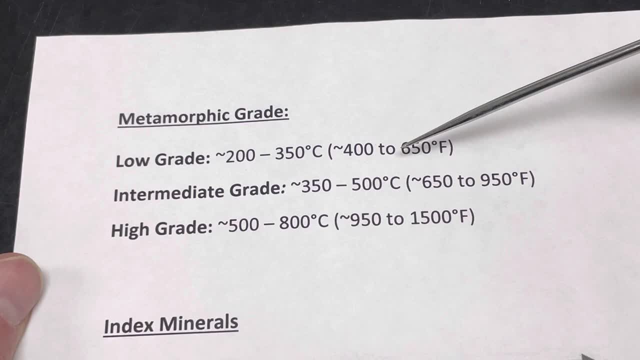 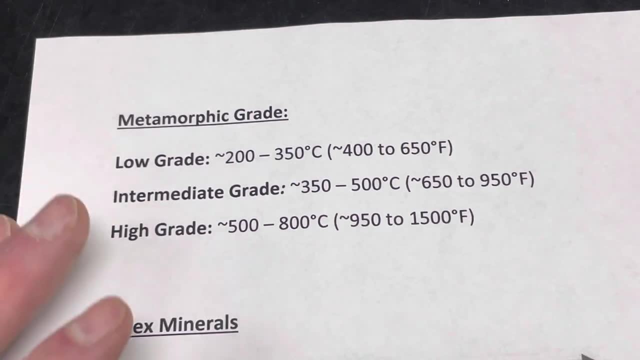 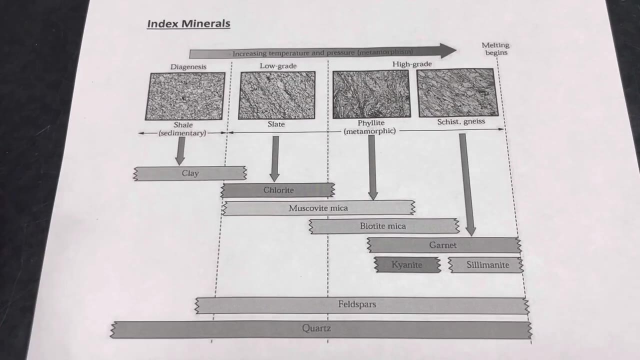 no idea how much, how, what kind of temperatures or pressures the rock was subjected to when it became a metamorphic rock, and to answer that, what we tend to use is this idea of index minerals. so what we have here- and i apologize, our color copier cut out this afternoon, so this is in- 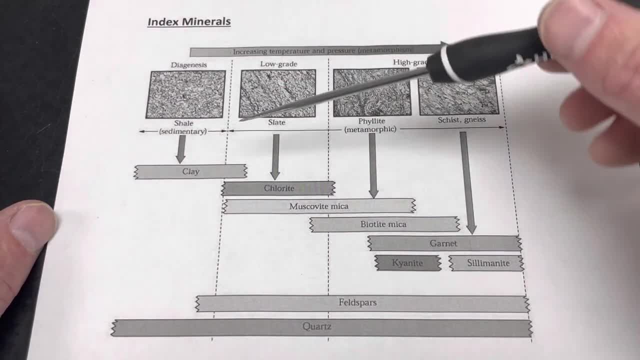 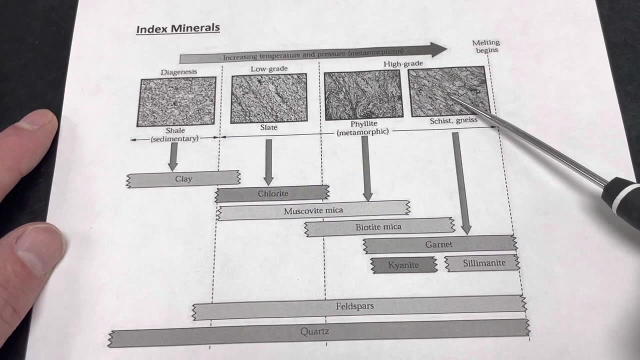 black and white. apologize, this is supposed to be in color, but what we have here is increasing temperature from left to right, so we can see low grade, more or less intermediate grade to high grade, and then we have a bunch of minerals, and we've covered some of these minerals in our 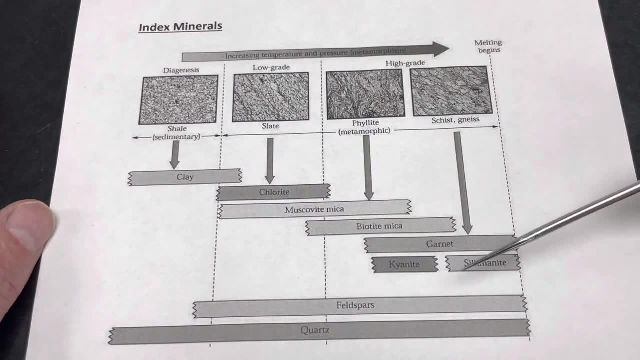 mineral series. so some of these you might be familiar with, like the quartz, the feldspars, biotite, muscovite. those are all minerals you may be familiar with, along with a few others. what this is showing us is that certain minerals- not every mineral, but many minerals- have a zone. 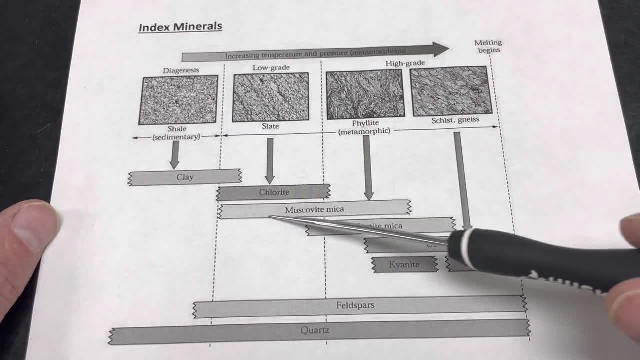 of temperatures in which they're stable, and so muscovite, for example, is going to be stable at low grade to intermediate grade metamorphic conditions. but as you increase the temperatures, muscovite will break down and start to form other minerals using those, those elements that 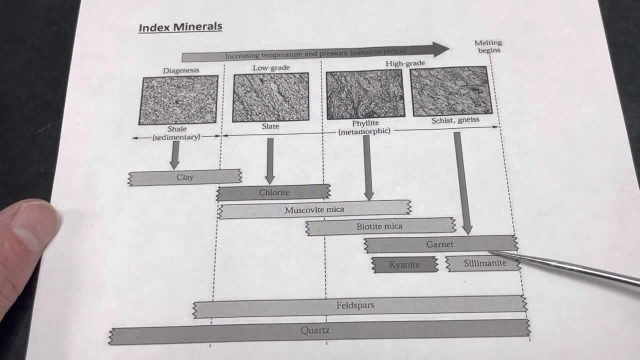 it's made out of notice that garnet or silimanite are associated with dominantly high grade metamorphism. these minerals are not going to show up or even form until the temperatures are quite a bit higher. some minerals, like quartz, don't help us at all because